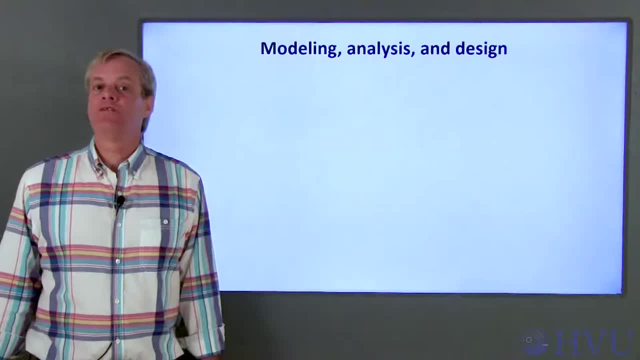 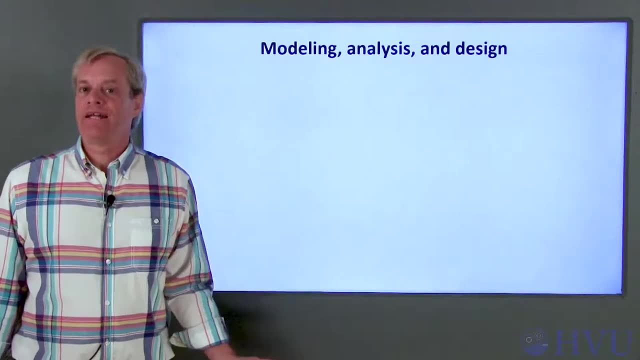 take a look at how modeling, analysis and design fit into an overall engineering process. This is important because we usually learn math in an environment where the mathematics itself is not designed to be a volume. The equations are to be about is of primary importance. 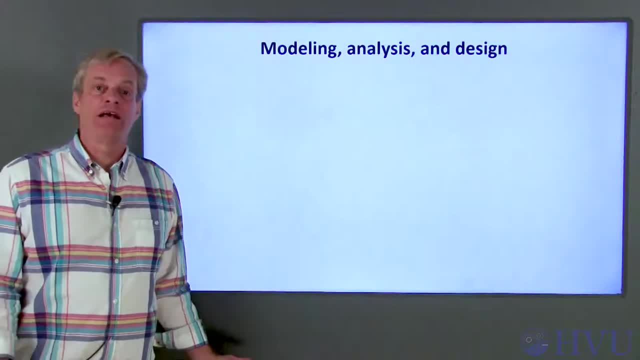 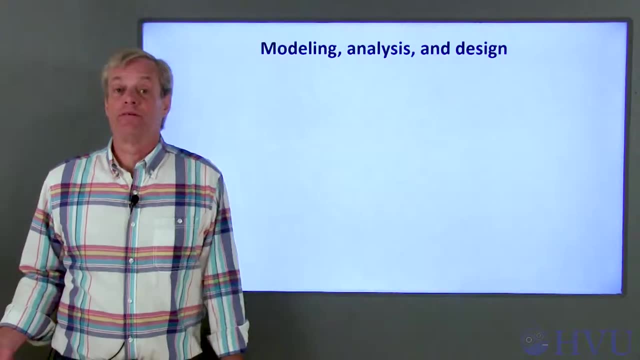 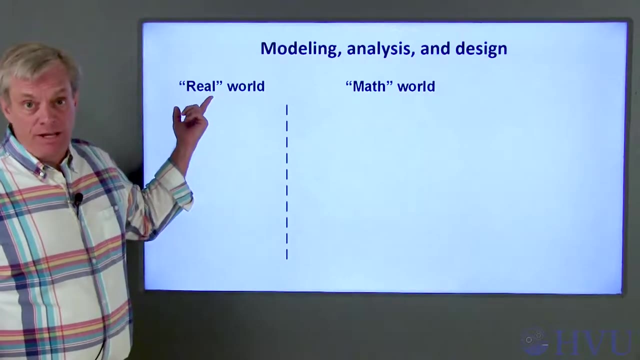 As engineers, the math is just a tool to help us understand the real world. There's kind of a fundamental difference between how engineers use math and how we're taught to use math. It's fundamental for engineers to work in two domains simultaneously. There's the real world of physical devices. 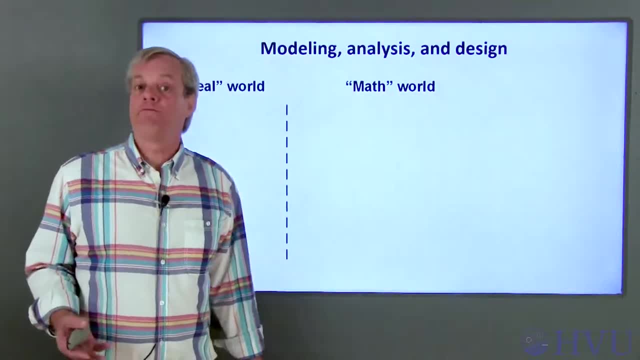 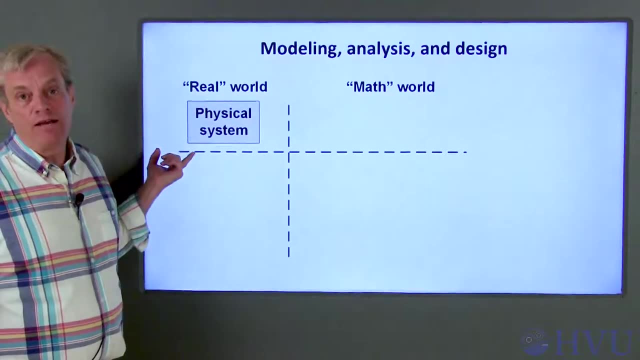 and the mathematical world, where we model the real world and quantify what's going on. The engineering process usually starts with at least some idea of what the physical system looks like. This might be a preliminary design. for example, We usually start by creating a mathematical model. 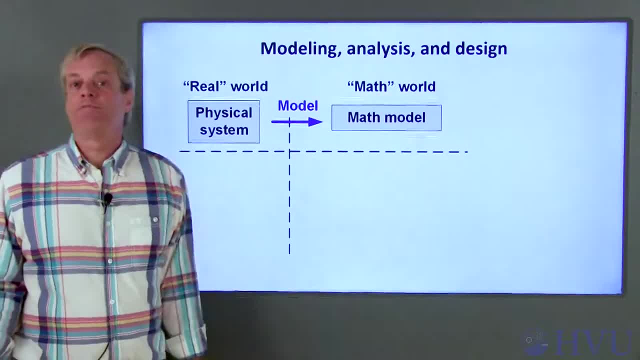 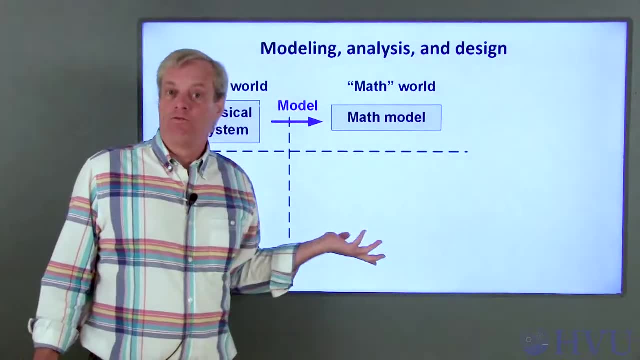 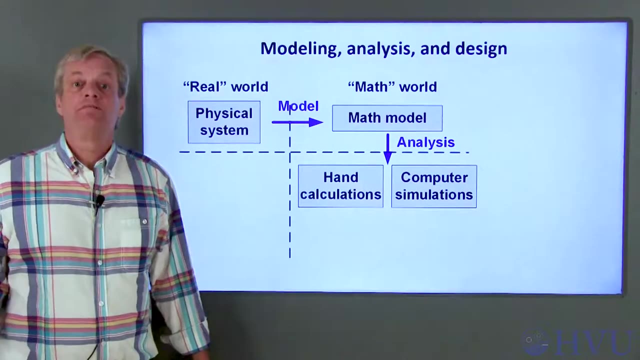 of this system. This model's also preliminary and it represents our first guess as to what we think will be important about this system. We're now in mathematics land rather than in the real world. In mathematics land we can analyze the system to see what we think the physical system will do. 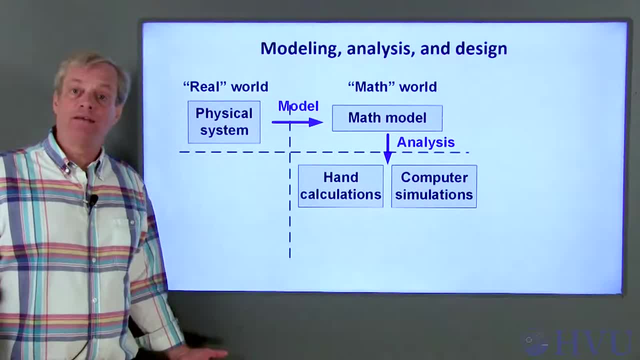 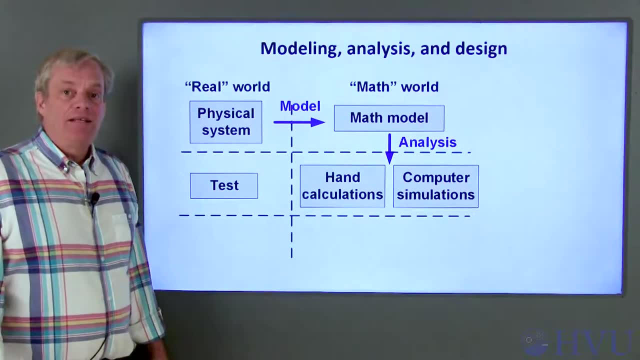 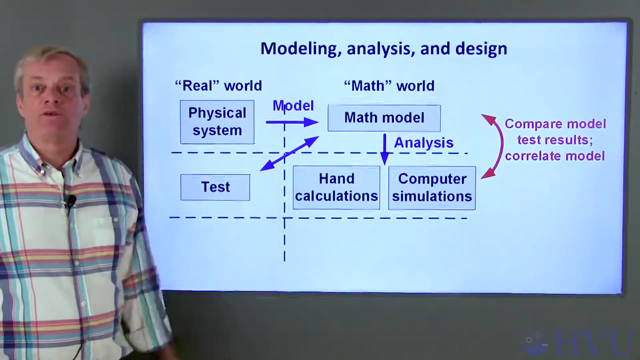 Depending on the complexity of the mathematical model, we can either do hand calculations to analyze the system or simulate the system response using a computer. We'll likely use the analysis and the preliminary design to build prototype hardware and test it. One huge benefit of this early testing. 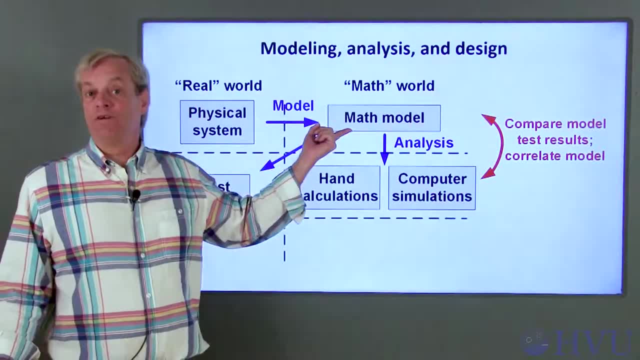 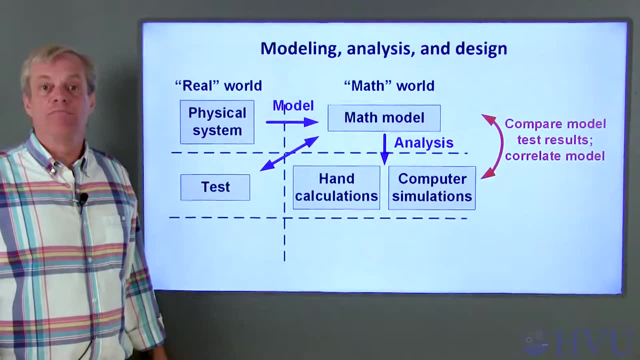 is to make sure that our mathematical models are actually predicting what's happening. So we'll probably test this system under conditions that we can analyze and modify our model as necessary to make the model agree with the test data. This process is called model correlation or validation. 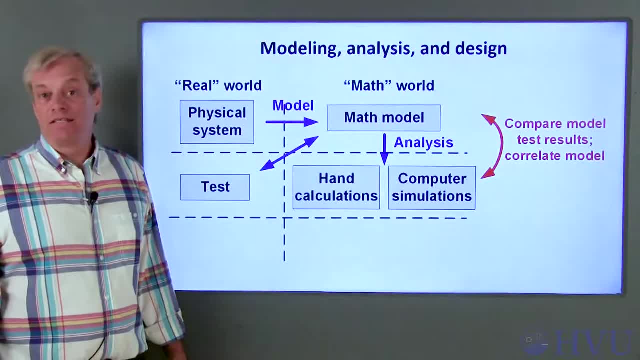 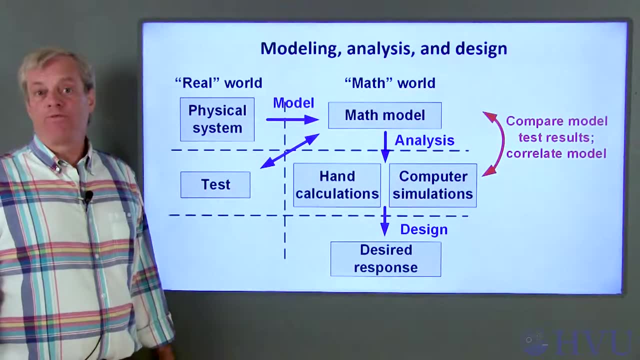 This step is crucial because we're going to use this model to finalize the system design and we don't want to use a model that doesn't reflect reality. Once we've got some confidence that the math we're using actually predicts reality, we can use the math model to modify this original design. 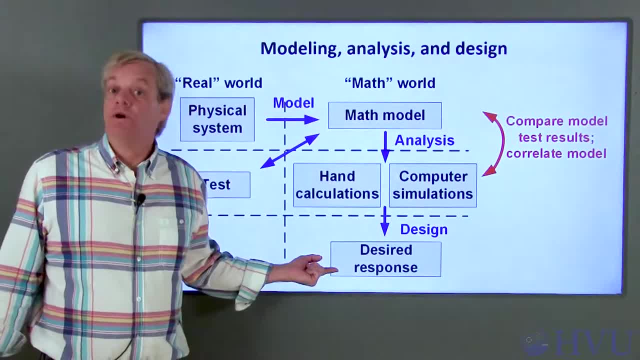 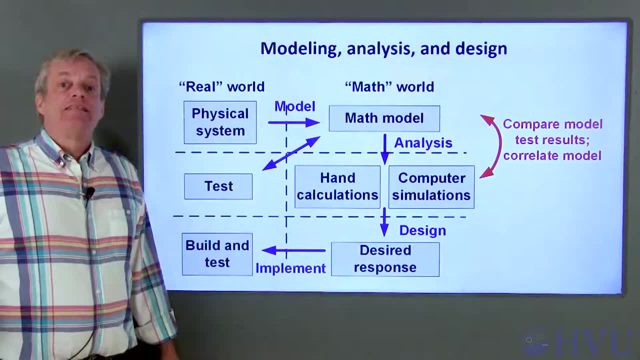 In this step, we know what kind of response we want from the system. We can now use our math model to evaluate what to change about the system to get that desired response. At this point we've got a new design that, on paper at least, does what it's supposed to do.